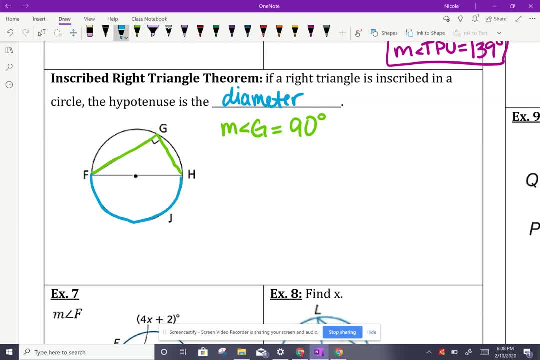 but this is a semicircle, Because if this is 90 degrees, if we're going from the inscribed to the arc, what do we do? What did we just talk about? we doing, us doing. we have to multiply by two, So that makes the measure of arc F J H equal to 180 degrees. So therefore, arc F J H. 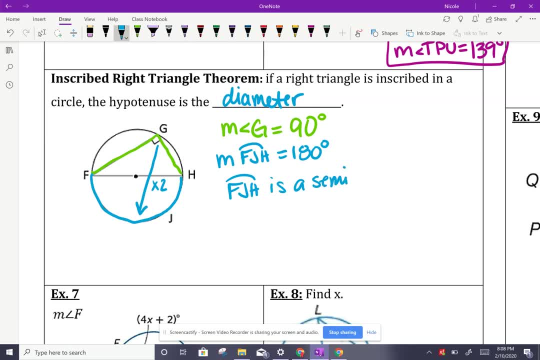 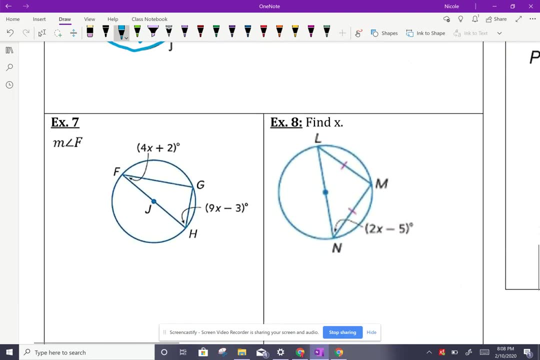 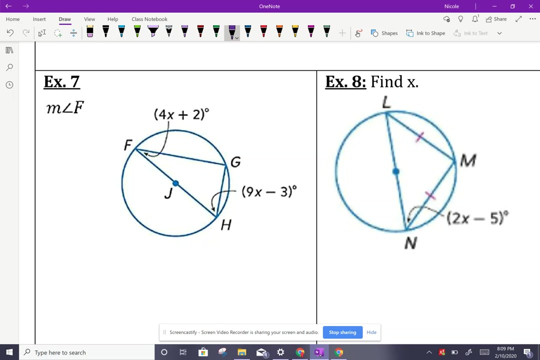 is a semicircle. Remember semicircle: half of the circle. the diameter cuts that circle in half, So we have a semicircle, For example, seven. I see that I have a triangle inscribed and that one side of that triangle is the diameter. So that means angle G is my right angle. 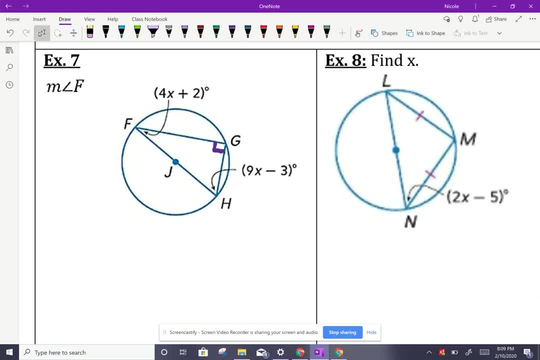 that is my right angle, So I need to solve for angle F. It's a right triangle. I know that I have 90. So a whole triangle is 90 as 180 degrees. So if I already know 90,, 180 minus 90 is 90,. 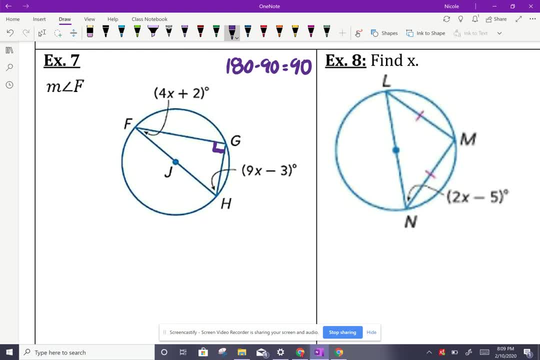 then F and H must add together to equal the other 90. So the measure of F plus the measure angle H equals 90 degrees. plug in all the pieces we have. we have four x plus two plus nine x minus three. 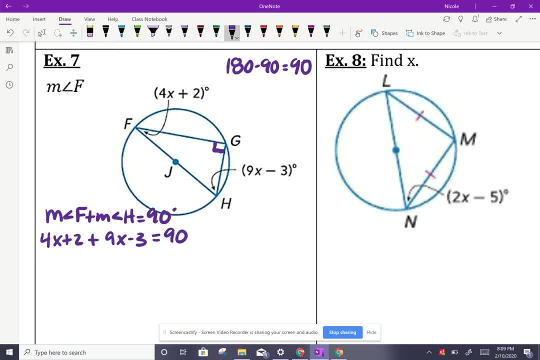 equals 90.. Combine your like terms: 13 x minus one equals 90.. 13 x equals 91. And so x is going to be equal to seven. Now it asks me to find the measure of angle F, So I need to plug that in. I have four times seven plus two. 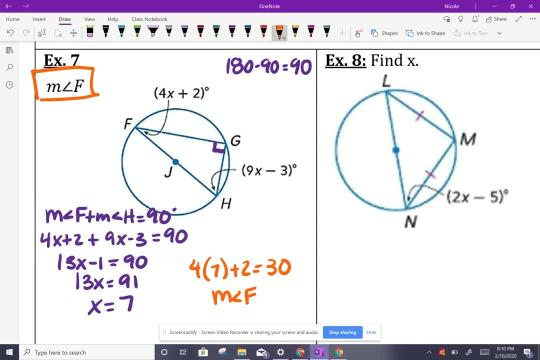 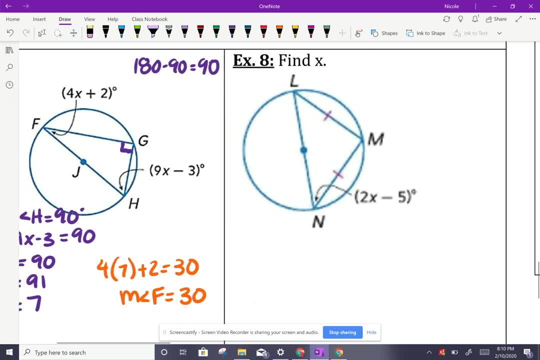 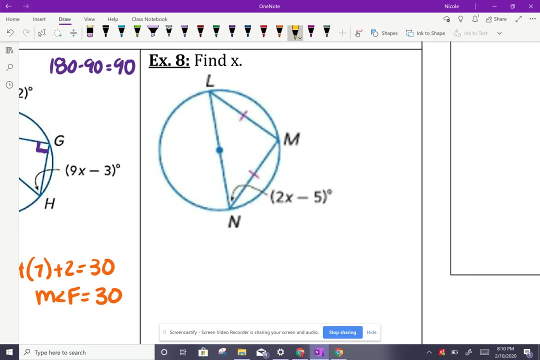 which is 30. So the measure of angle F equals 30. We have another example. We have another triangle inscribed into our circle with one side being the diameter. So that means angle M is a right angle. It also tells me this is isosceles.